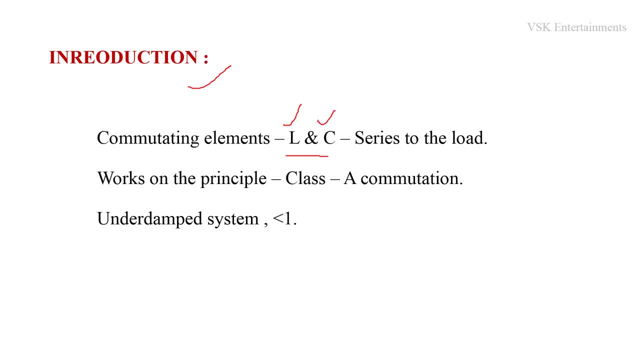 storage elements, that is, inductor and capacitor, The inverters in which inductor and capacitor are connected in series to the load. Those type of inverters are called series inverters, Coming to working principle of series inverter. The working principle of series inverter is: 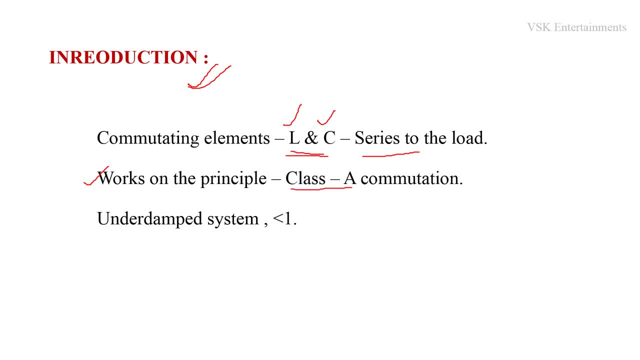 depends upon the class A commutation. That is, class A commutation is nothing. but this is the one of the type of the forced commutation. The working of series inverter is depends upon this class A commutation. Similarly, here the commutating elements and load forms the under damped system. 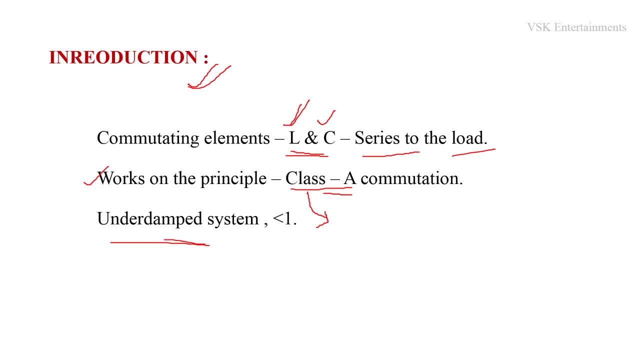 Under damped system is nothing but in which the damping factor of the system is less than unity of series inverter, that is, the commutating elements are connected in series to the load and it works on the class, a commutation principle, and it forms the underdamped system. 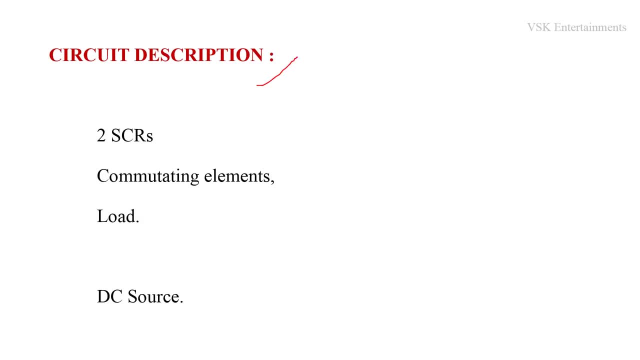 coming to circuit description of series inverter, it consisting of two acrs commutating elements. those are nothing but inductor and capacitor and load. this entire thing is supplied by the dc voltage source. this is the circuit diagram of series inverter. in this we are raising two. 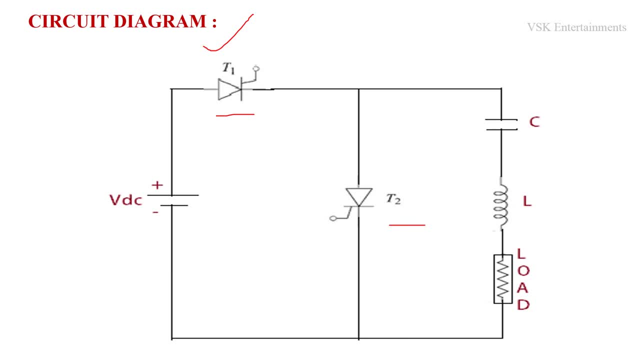 thyristors t1, t2 and commutating elements, inductor and capacitor and load. here these commutating elements are connected in series to the load and this entire circuit is supplied by the constant voltage source, vdc. here the working of series inverter depends upon the class a. 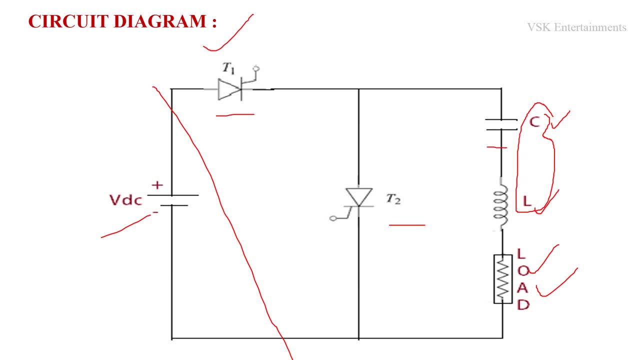 commutation, that is nothing, but by using the voltage acrs. commutation, that is nothing. but by using the voltage acrs. commutation, that is nothing but across this capacitor, we are going to turn off the main thyristor t1, then we are going to get the 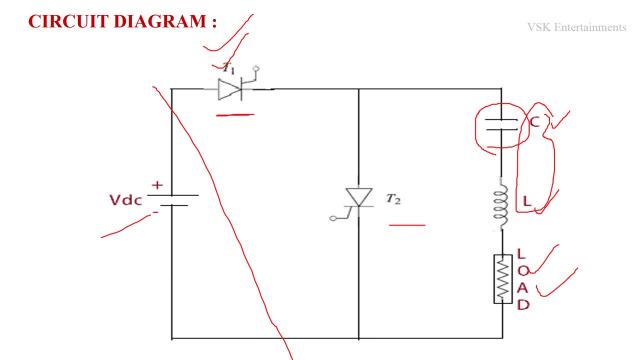 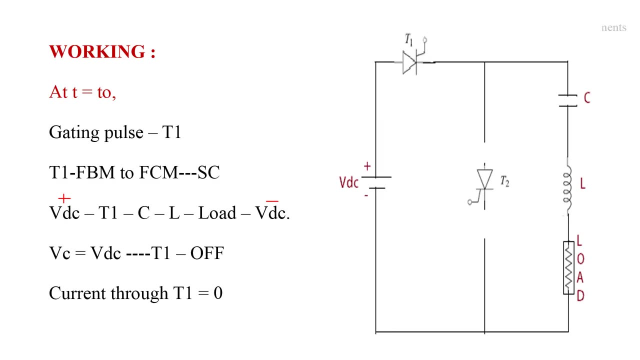 ac voltage. that's the working principle of class a, commutation, as well as series inverter. now we are going to discuss about working of series inverter. coming to working, the concept of working of series inverter is very simple. listen carefully. that is by applying the constant. 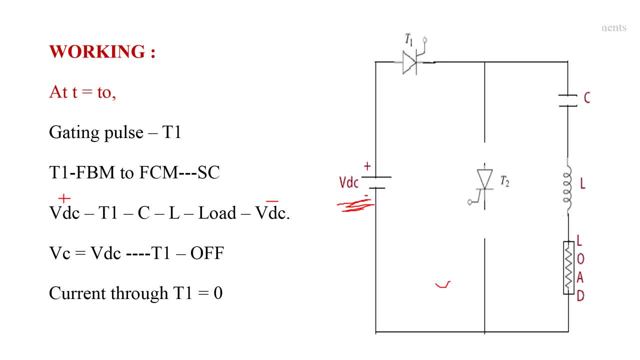 voltage source to the circuit. thyristors t1 is in forward blocking mode and thyristor t2 is in forward blocking mode without applying the gating pulses to these two thyristors. both the thyristors act as a open circuit. there is no path for current from source to load now at time. 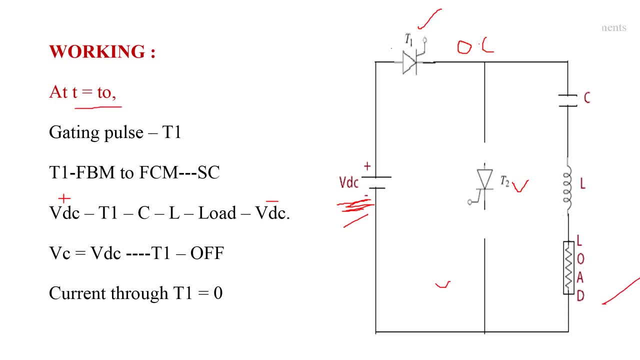 t is equal to t naught. we are going to apply the gating pulse to thyristor t1. by applying the gating pulse to thyristor t1, thyristor t1 comes from forward blocking mode to forward conducting mode and it act as a short circuit. 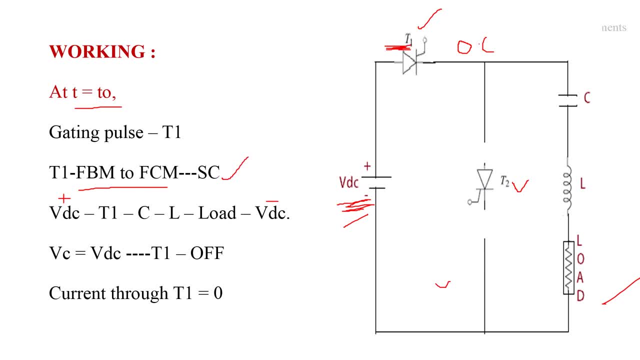 circuit and it allows the flowing of current from source to load in the direction of vdc plus, thyristor t1, capacitor inductor load and vdc minus. that is nothing but in this path. and here capacitor starts charging, with upper plate as positive and lower plate as negative, whenever. 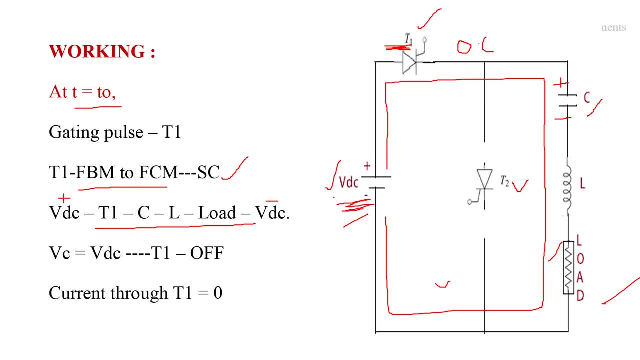 this capacitor charges to the voltage vdc, that is nothing. but whenever vc is equal to vdc, the potential difference between this capacitor and this voltage is zero. if potential difference is zero, there is no path for current from this point, and this point means the current flowing. 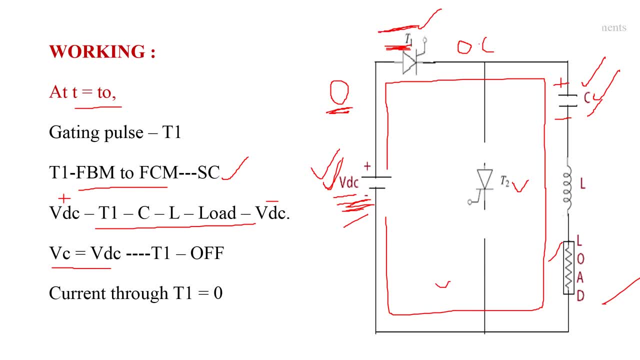 through thyristor t1 becomes zero. whenever current flowing through thyristor t1 becomes zero, the current flowing through thyristor t1 becomes zero, the current flowing through thyristor t1 comes to off state, comes to off state. that is nothing at class a commutation. that is whenever. 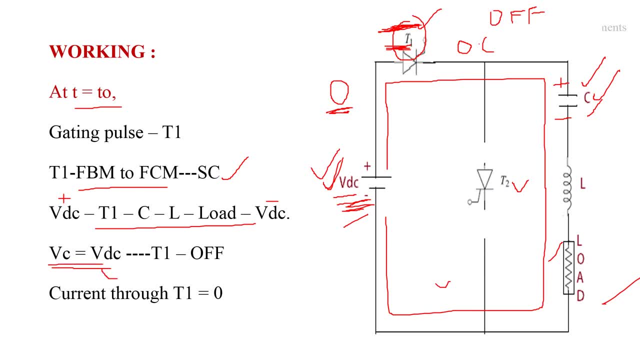 vc is equal to vdc, the current flowing through thyristor t1 becomes zero. why? because the potential difference between vdc and capacitor c is zero, so the current flowing through thyristor t1 becomes zero. if current flowing through thyristor t1 becomes zero, thyristor t1 automatically comes. 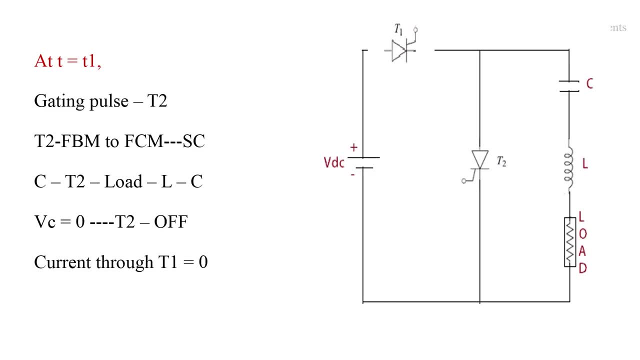 comes into half state. in previous case, capacitor c is charges with upper plate as positive and lower plate as negative and it having the voltage v d c okay. whenever v c is equal to v d c, the current flowing through thyristor t 1 is 0 and thyristor t 1 comes into half state. now in this, 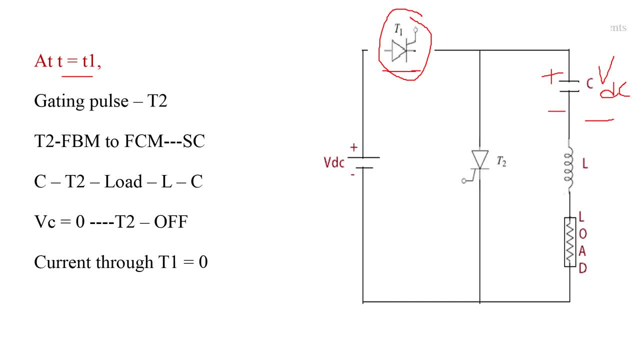 case, at time t is equal to t 1. we are going to apply the gating pulse to thyristor t 2. due to the application of gating pulse to thyristor t 2. thyristor t 2 comes from forward blocking mode to. 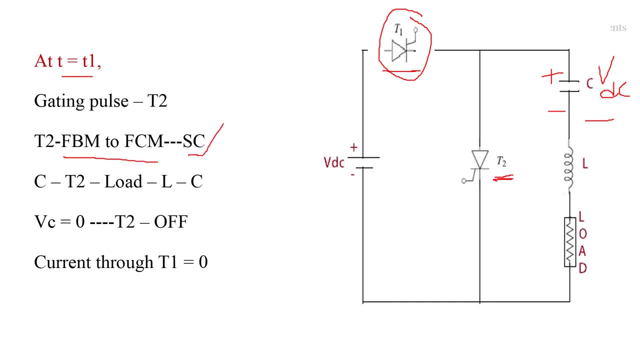 forward conducting mode and it act as a short circuit due to the short circuit of thyristor t 2. here capacitor starts discharging in the direction of c plus, thyristor t 2, load inductor and and and c minus. that is nothing but in this direction. here c is nothing but c plus and here c is nothing. 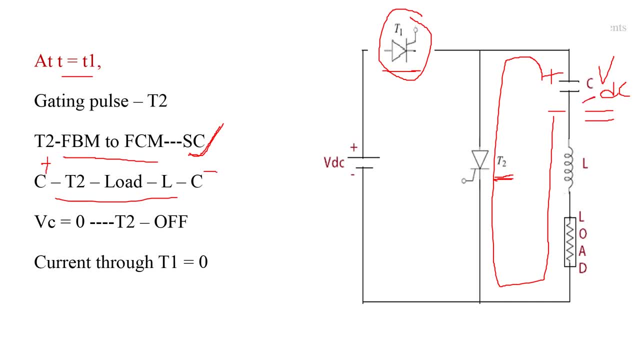 but c minus. after complete discharging of this capacitor, that is nothing. but whenever v c is equal to 0, capacitor changes its polarities, that is, upper plate as negative and lower plate as positive, and the current flowing through thyristor t 2 becomes 0. whenever current flowing through thyristor t 2 becomes 0 means 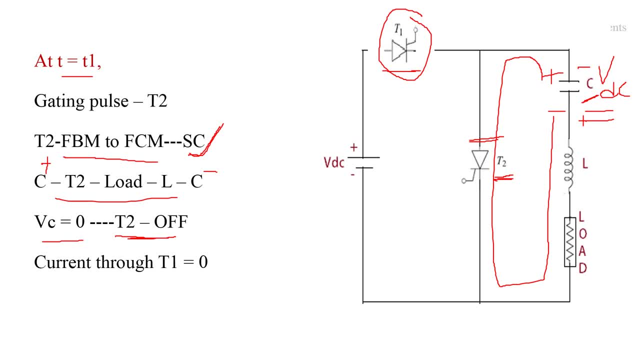 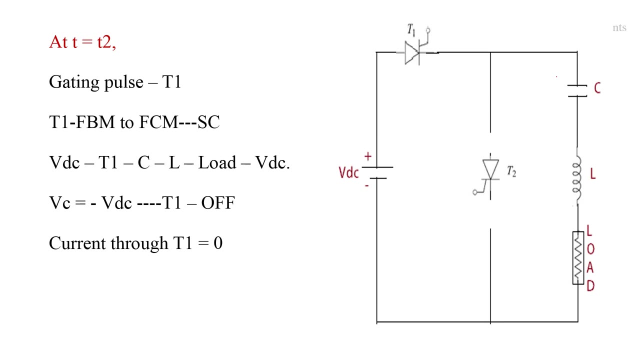 thyristor t 2 comes into half state. here there is no path for current from source to load. that is nothing but the current flowing through. thyristor t 1 is 0 in previous case, after complete discharging of capacitor, capacitor changes its polarities, that is, upper plate as negative and lower plate as 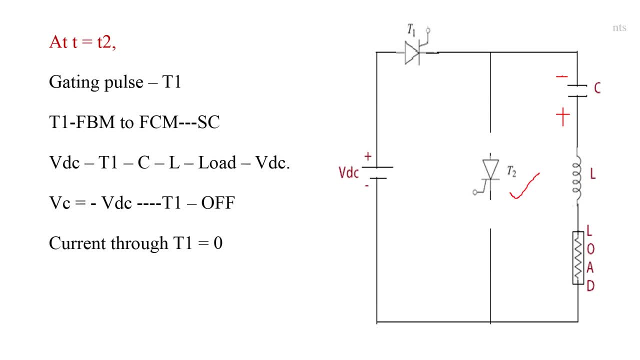 positive and thyristor t 2 comes into half state. in this case, at time t is equal to t 2. again, we are going to apply the gating pulse to thyristor t 2. and we are going to apply the gating pulse to thyristor t 2 and we are going to apply the gating pulse to thyristor t 1 by applying the gating pulse. 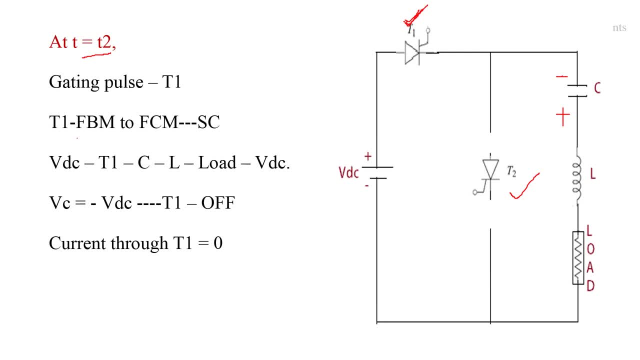 to thyristor t 1. thyristor t 1 comes from forward blocking mode to forward conducting mode and it act as a short circuit and it allows the flowing of current from source to load in the direction of vdc. place thyristor t 1: c l load and vdc minus. that is nothing but in this direction. here vdc is vdc. 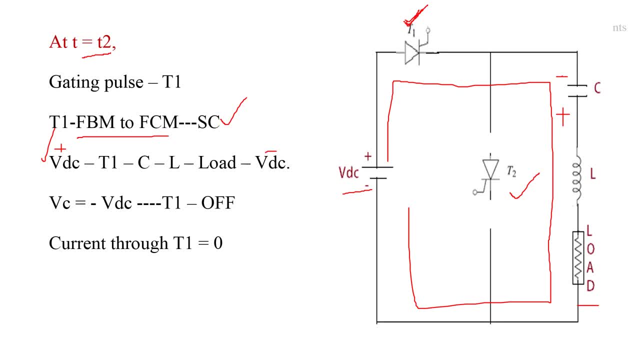 place and vdc minus. in this case also capacitor starts charging up to the voltage vdc, but in opposite direction due to the opposite polarities. whenever this capacitor charges up to the voltage minus vdc, again, thyristor t 1 comes into half state. when thyristor t 1 is in half state, the 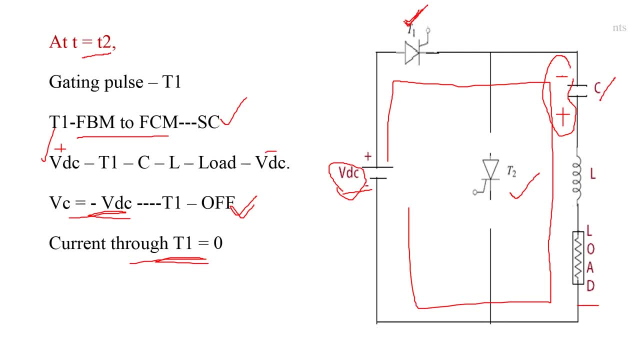 current flowing through thyristor t 1 becomes 0 again, we are going to apply the gating pulse to thyristor t 2. by applying the gating pulse to thyristor t 2, again capacitor starts discharging. after complete discharging of capacitor c, again capacitor c changes its polarities. again we are 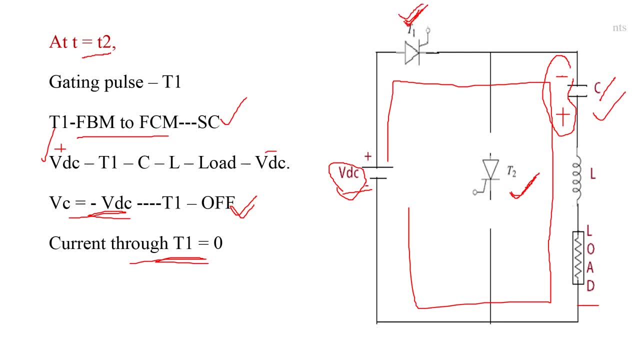 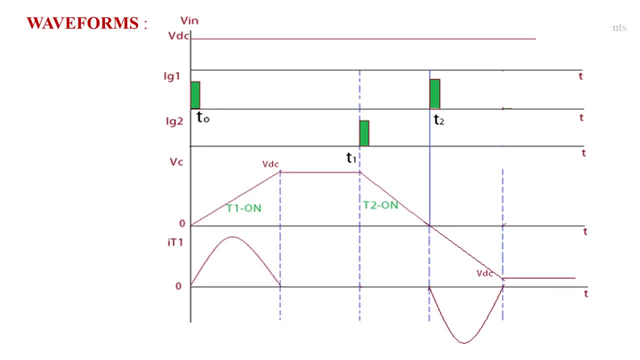 going to apply the gating pulse to thyristor t 1, same cycle going to repeats. by using this analysis, we are going to draw the waveforms. these are the waveforms, depending upon the above analysis. here v n is the constant dc voltage source, ig 1 and. 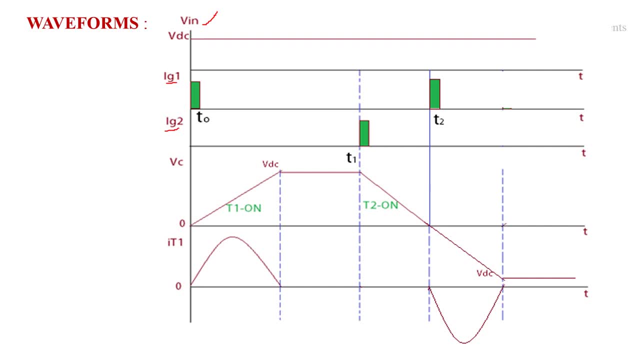 ig 2 are the gating pulses which we are going to apply to the thyristor t 1 and t 2, and vc is the voltage across capacitor and it 1 is the current flowing through thyristor t 1. initially, at time, t is equal to t naught. we are going to apply the gating pulse to thyristor t 1 due to 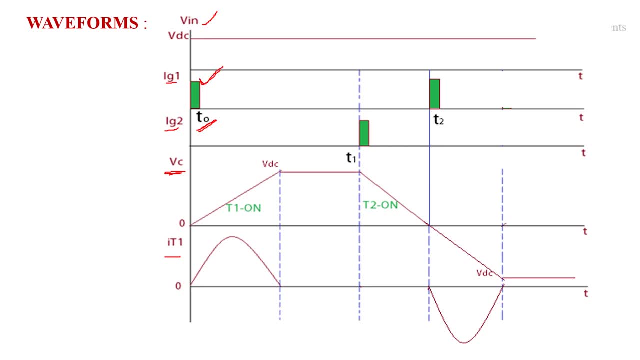 the application of thyristor t 1. thyristor t 1 comes from forward blocking mode to forward conducting mode and capacitor starts charging means the voltage across capacitor is increases voltage vdc. whenever the voltage across capacitor reach to the voltage vdc, the current flowing 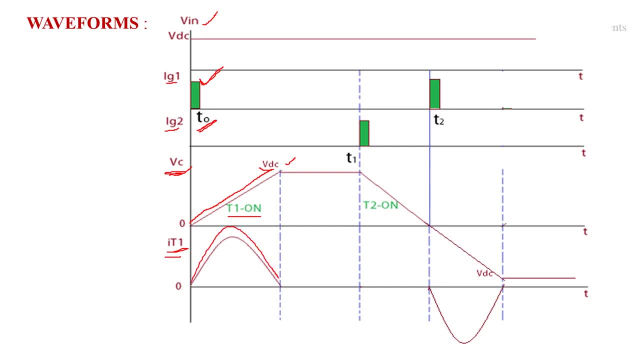 through thyristor t1 comes to 0. whenever current flowing current flowing through thyristor t1 comes to 0, t1 comes into off state means in this duration the voltage across capacitor is plus vdc and thyristor t1 is in off state means the current flowing through thyristor t1 is. 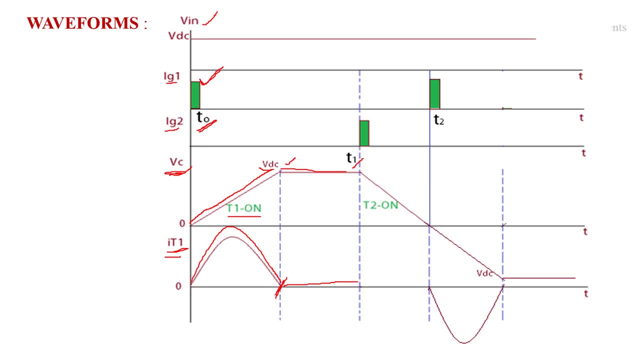 0. again. at time t is equal to t1. we are going to apply the gating pulse to thyristor t2. due to the application of gating pulse to thyristor t2, capacitor starts discharging, that is, capacitor starts discharging from vdc plus to 0 in this duration. also, thyristor t1 is in off state. 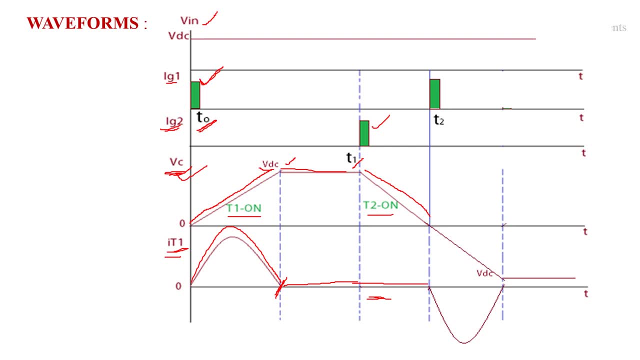 so the current flowing through thyristor t1 is 0 after complete discharging of thyristor. after complete discharging of capacitor, thyristor t2 comes into off state again. at time t is equal to t2. we are going to apply the gating pulse to thyristor t1 again. due to the application of gating pulse to thyristor t1.